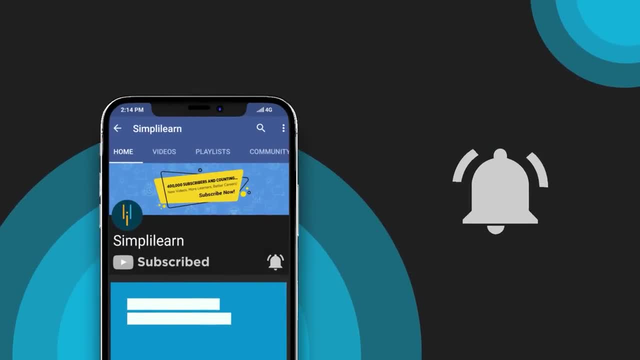 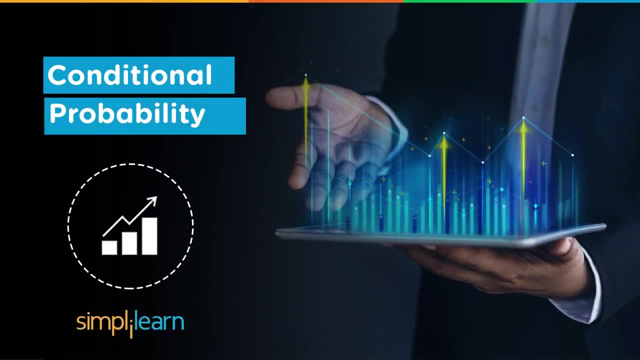 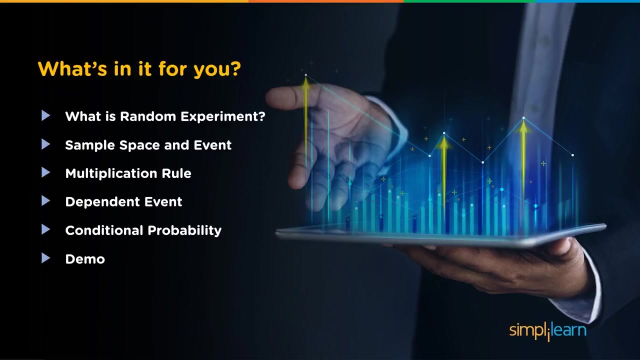 Hi everyone, Welcome to this exciting session by Simply Learn. Today, we have a really interesting topic for you. In this video, we'll be discussing conditional probability, which is one of the most important areas in probability theory. We'll start by talking about random experiments. 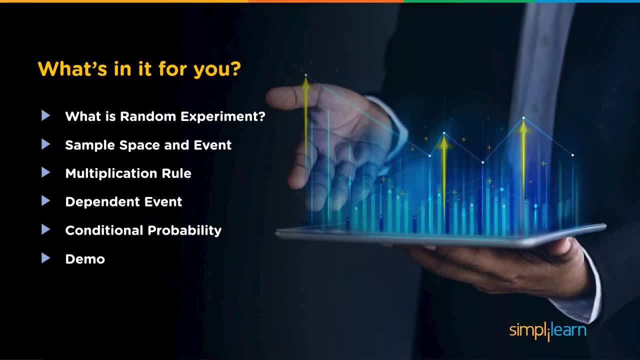 and then move on to events and sample space. Then we'll try to understand the multiplication rule with the help of an example. After that, we'll learn about dependent events and the multiplication rule associated with them. After that, we'll learn about conditional 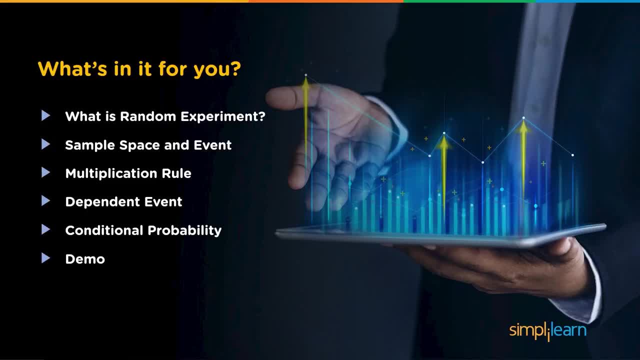 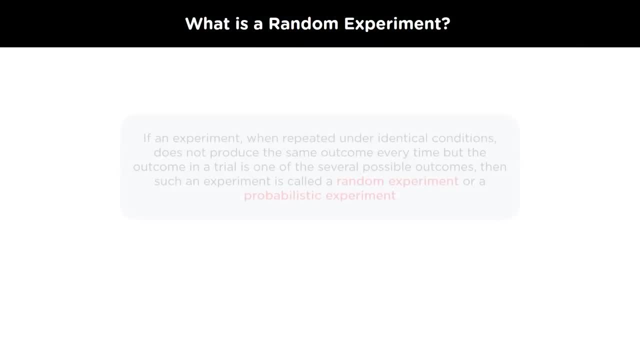 probability with the help of an example. So let's get started. What is a Random Experiment? Lets say that you roll a fair die and there are 6 possible outcomes. You can get a number from 1 to 6, but it is impossible to assume. 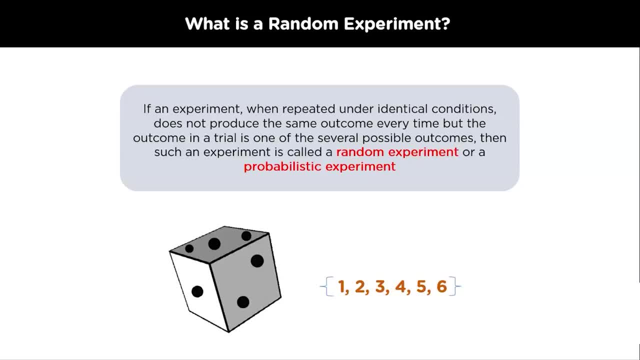 accurately predict the outcome. In mathematical theory, we consider only those experiments or observations for which we know the set of possible outcomes. Also, it is important that predicting a particular outcome is impossible. Such an experiment, where we know the set of all the possible results but find it impossible to predict any one particular execution, is 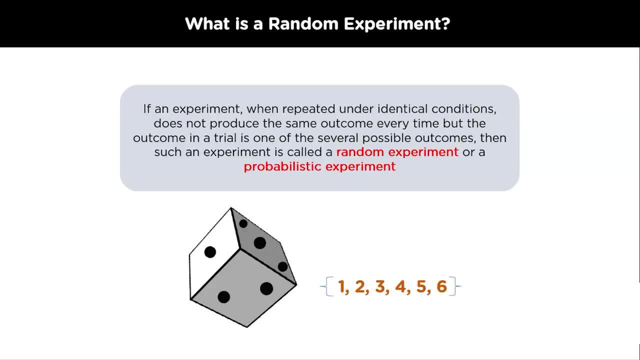 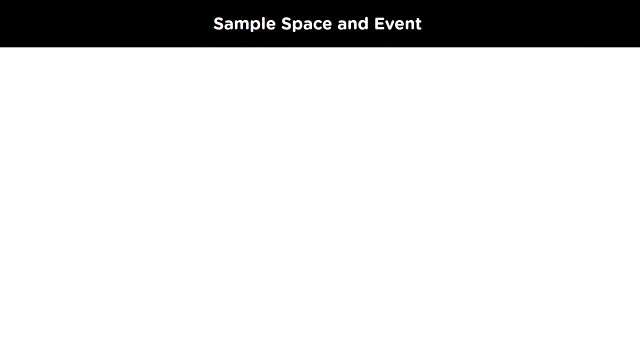 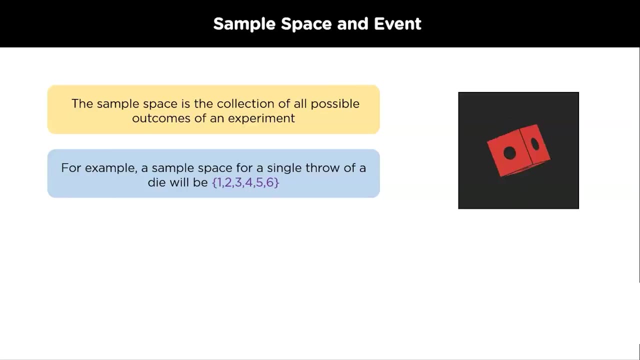 a random experiment. Even if a random experiment is repeated under identical conditions, the outcomes or results will fluctuate randomly. Sample Space and Events. The sample space associated with a random experiment is the set of all the possible outcomes. Suppose you roll a die, so the sample space for a single throw up die will be 1,. 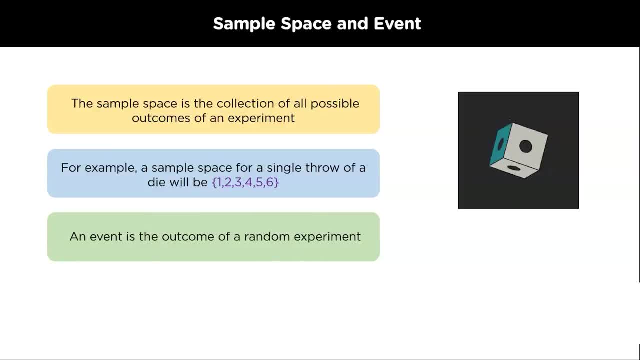 2, 3,, 4, 5 and 6.. An event is a subset of the sample space, or you can say it is an outcome of a random experiment. Getting a hit when we toss a coin is an event. Now we will discuss about multiplication rule. in probability, The multiplication rule says: 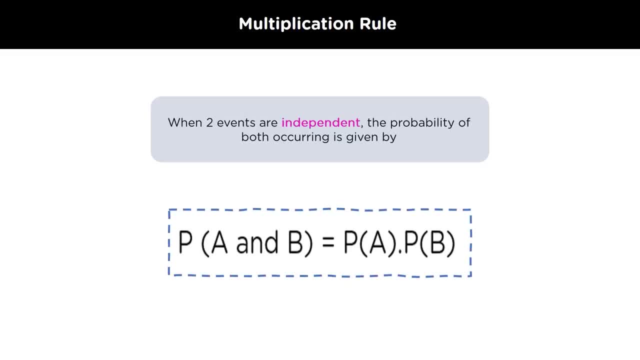 that events are independent. the probability of both occurring simultaneously is given by probability of A. intersection B will be equal to probability of A into probability of B. Let's understand this with the help of an example. If a coin is tossed twice, what will? 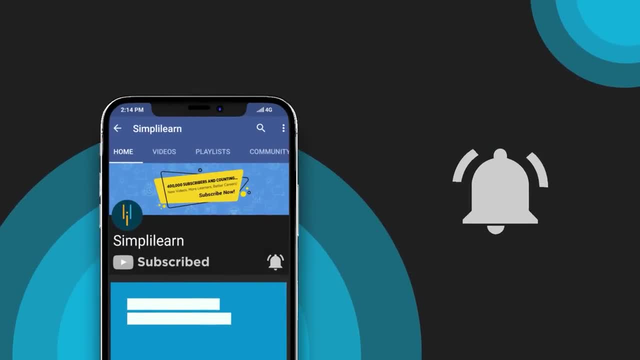 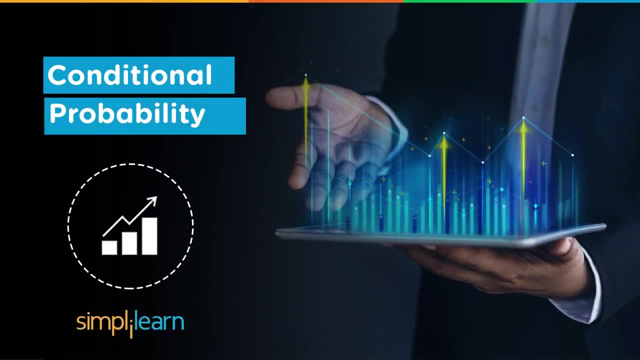 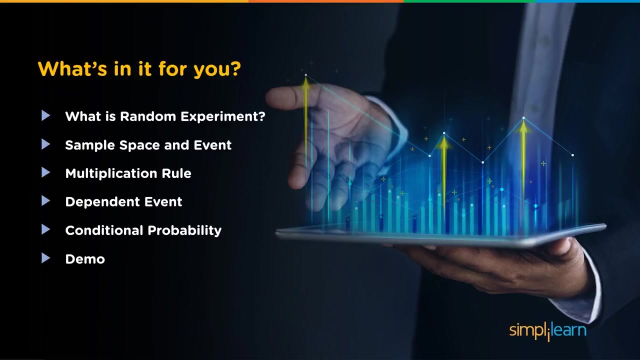 Hi everyone, Welcome to this exciting session by Simply Learn. Today, we have a really interesting topic for you. In this video, we'll be discussing conditional probability, which is one of the most important areas in probability theory. We'll start by talking about random experiments. 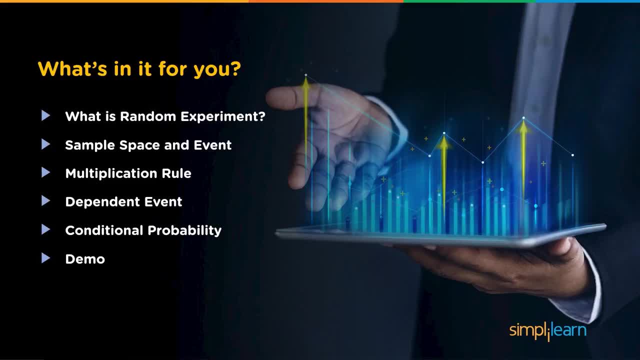 and then move on to events and sample space. Then we'll try to understand the multiplication rule with the help of an example. After that, we'll learn about dependent events and the multiplication rule associated with them. After that, we'll learn about conditional 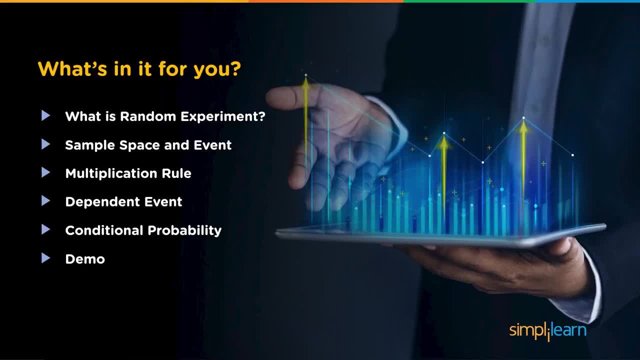 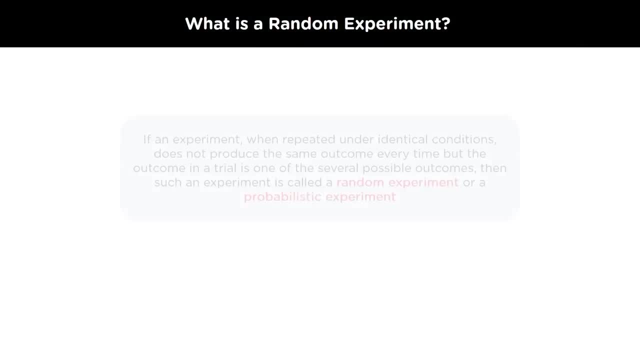 probability with the help of an example. So let's get started. What is a random experiment? Let's say that you roll a fair die and there are six possible outcomes. You can get a number from one to six, But it is impossible to understand. So 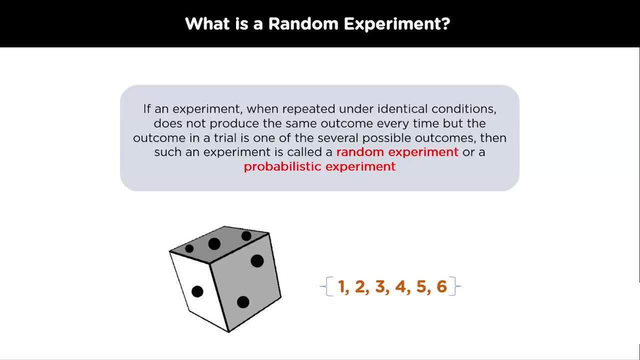 accurately predict the outcome. In mathematical theory, we consider only those experiments or observations for which we know the set of possible outcomes. Also, it is important that predicting a particular outcome is impossible. Such an experiment, where we know the set of all the possible results but find it impossible to predict any one particular execution, is 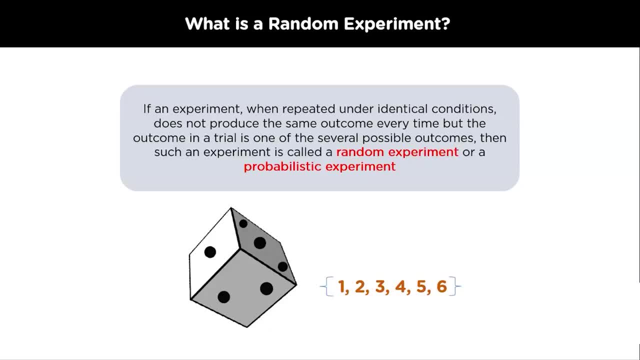 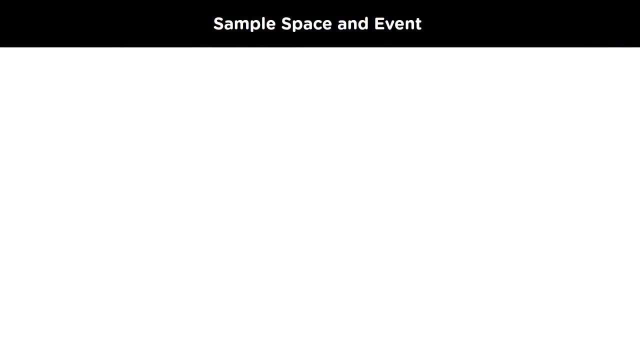 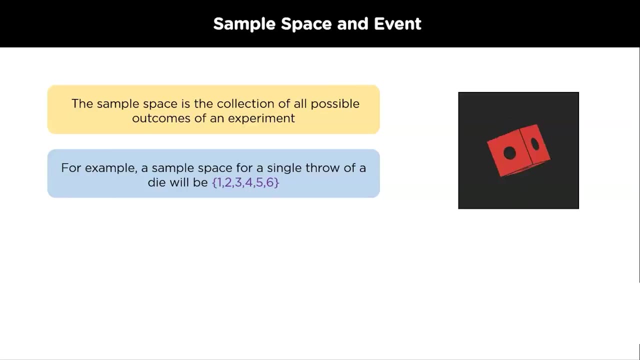 a random experiment. Even if a random experiment is repeated under identical conditions, the outcomes or results will fluctuate randomly. Sample space and Events. The sample space associated with a random experiment is the set of all the possible outcomes. Suppose you roll a die, So the sample space for a single throw-up die will be 1,. 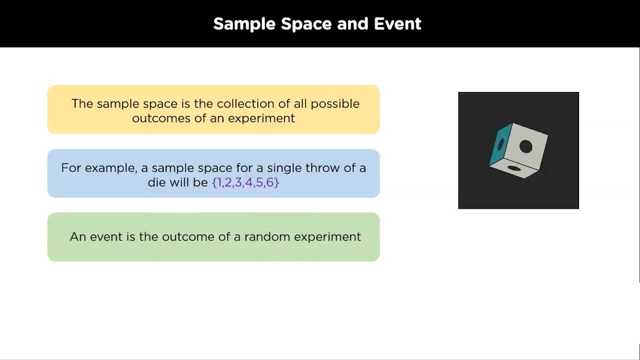 2, 3,, 4, 5 and 6.. An event is a subset of the sample space, or you can say it is an outcome of a random experiment. Getting a heads when you toss a coin is an event. Now we will discuss about the multiplication rule in probability. The multiplication rule. 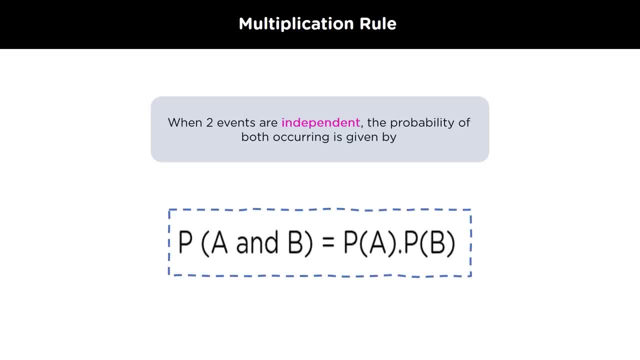 says that When two events are independent, the probability of both occurring simultaneously is given by probability of A. intersection B will be equal to probability of A into probability of B. Let's understand this with the help of an example. If a coin is tossed twice, what will? 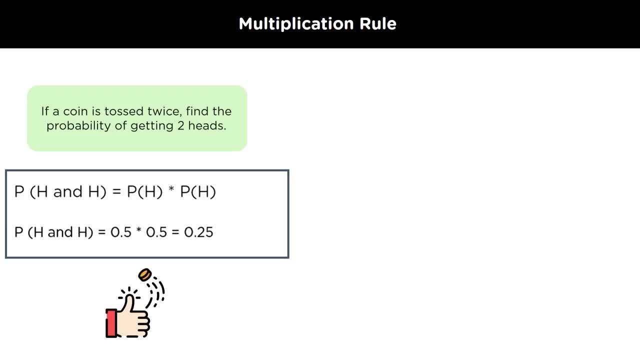 be the probability of getting two heads. So in a single throw the probability of getting a heads is 1 by 2, that is 0.5.. So the probability of getting the two heads in both the coins will be 0.5 into 0.5, which will be equal to 0.25.. Let's look at another example. Suppose 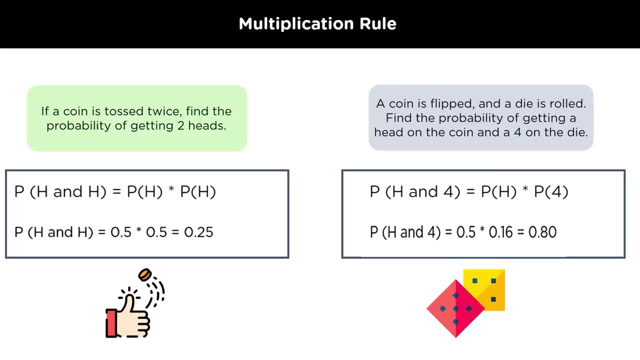 a coin is flipped and a die is rolled at the same time. So what will be the probability of getting a head on the coin and 4 on the die? So the probability of getting a heads, as discussed in the previous example will be- is equal to 0.5 and the probability of 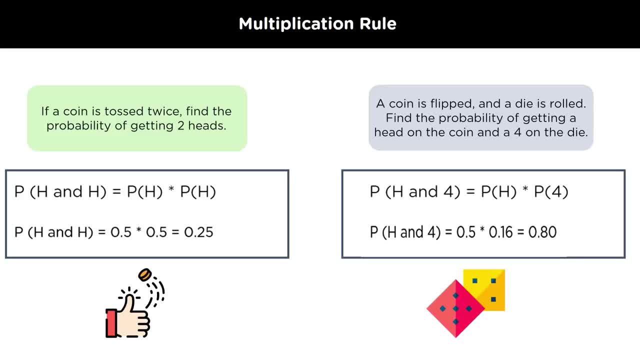 getting a 4 on a single throw of die will be 1 by 6, since there are 6 samples faced and 1 favorable outcome. So the probability of getting a heads will be 0.5 and the probability of getting a head on a coin and 4 on a die will be is equal to 0.5 x 0.16, which will 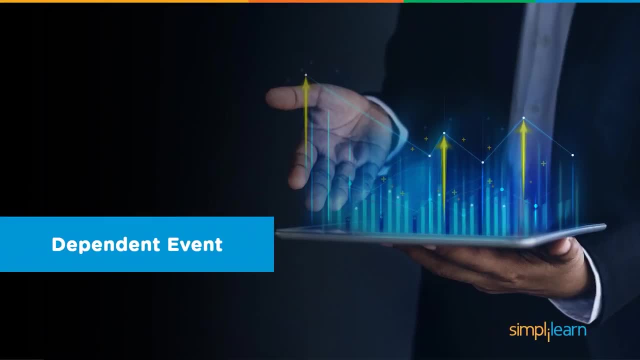 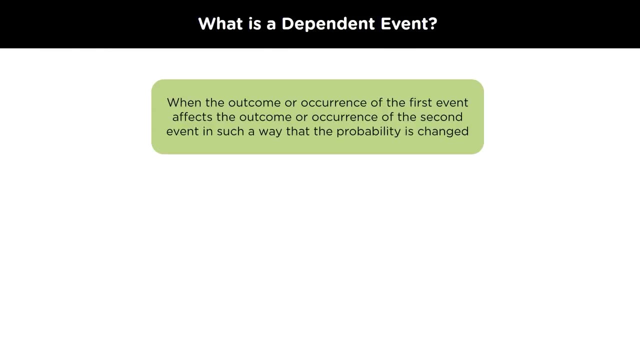 come out to be 0.80.. Now let's move on to dependent events. 2. events are said to be dependent if the outcome of the first event affects the outcome of the second event, so that the probability is changed. Let's understand this with the help of an example. Suppose: 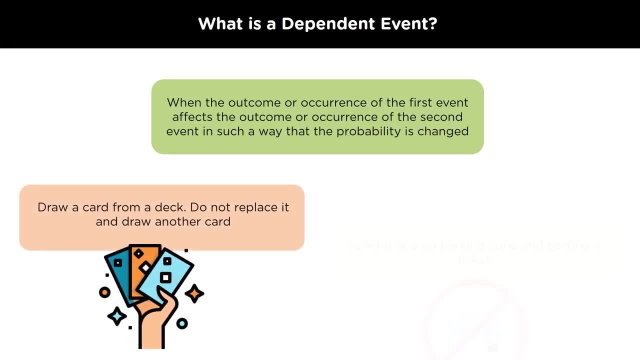 you have a deck of cards. The probability of drawing a card from a deck of cards is 1x52.. Now, if you do not replace the card, the probability of drawing other card changes to 1x51.. Another example of it can be a parked, no parking zone and getting a ticket When 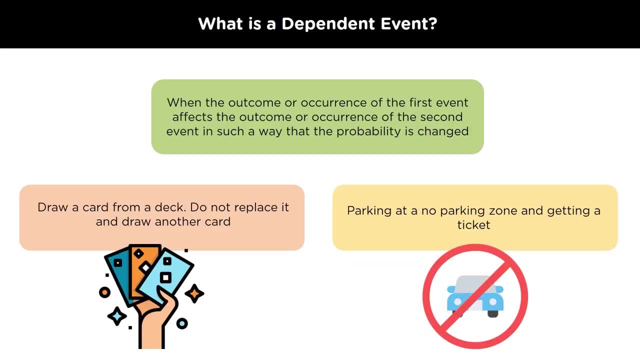 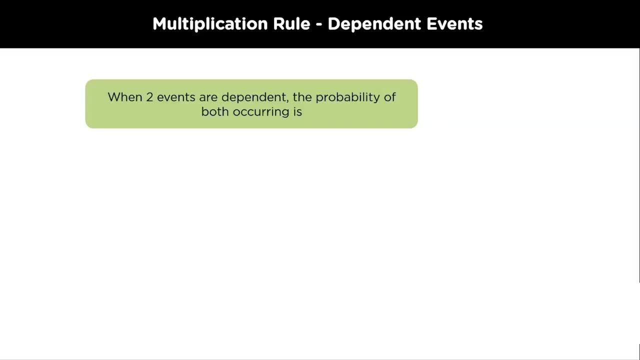 you park at a no parking zone, the probability of getting a ticket increases. There is a multiplication rule needs to be done for dependent events. It says that when two events are dependent, the probability of both occurring is given by this formula, which is P- A intersection. 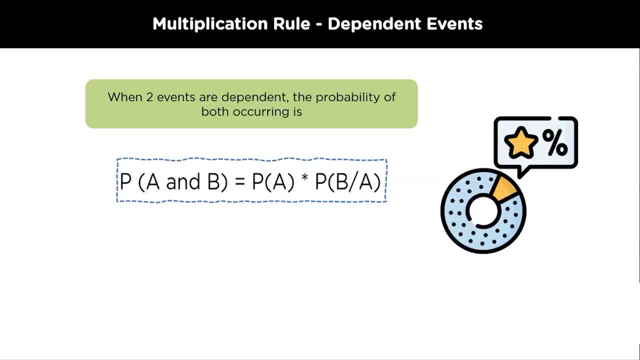 B is equal to P. probability of A into probability of B slash A. The slash reads the probability that B occurs, given that A has already occurred. Let's look at an example. Three cards are drawn from a deck and are not replaced. What would be the probability? 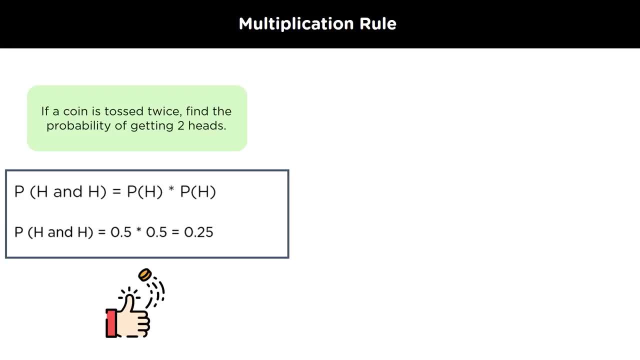 be the probability of getting two heads. So in a single throw the probability of getting a heads is 1 by 2, that is 0.5.. So the probability of getting the two heads in both the coins will be 0.5 into 0.5, which will be equal to 0.25.. Let's look at another example. Suppose 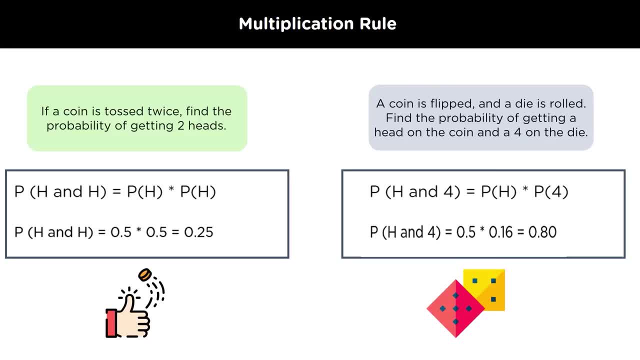 a coin is flipped and a die is rolled at the same time. So what will be the probability of getting a head on the coin and 4 on the die? So the probability of getting a heads, as discussed in the previous example will be- is equal to 0.5 and the probability of 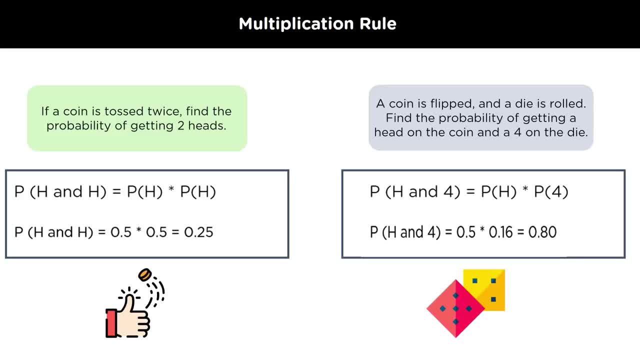 getting a 4 on a single throw of die will be 1 by 6, since there are 6 samples faced and 1 favorable outcome. So the probability of getting a heads will be 0.5 and the probability of getting a head on a coin and 4 on a die will be is equal to 0.5 x 0.16, which will 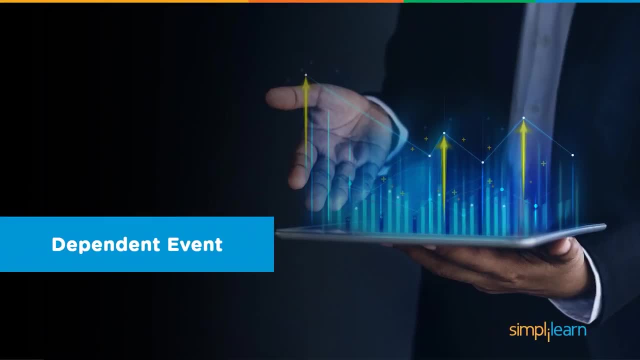 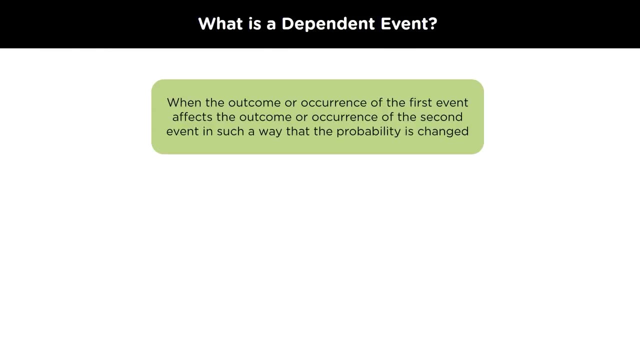 come out to be 0.80.. Now let's move on to dependent events. 2. events are said to be dependent if the outcome of the first event affects the outcome of the second event, so that the probability is changed. Let's understand this with the help of an example. Suppose: 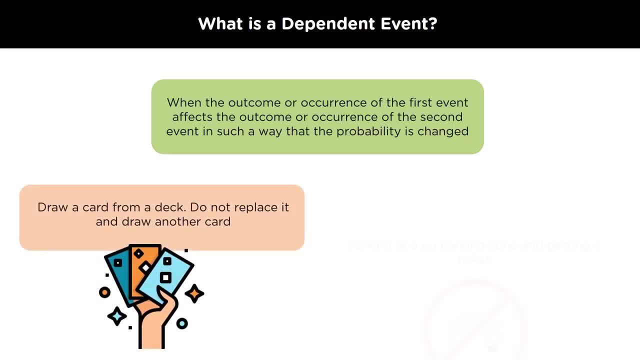 you have a deck of cards. The probability of drawing a card from a deck of cards is 1 by 52. Now, if you do not replace the card, the probability of drawing another card changes to 1 by 51.. Another example of it can be parking at a no parking zone and getting a ticket. 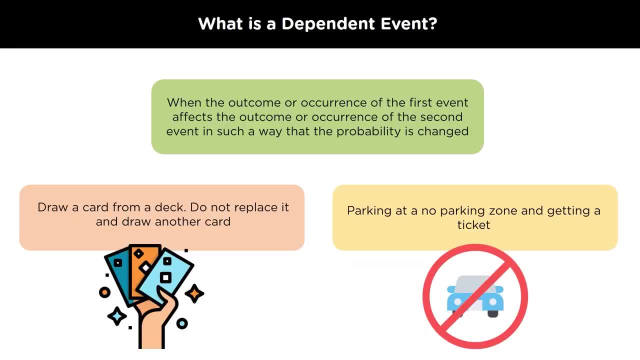 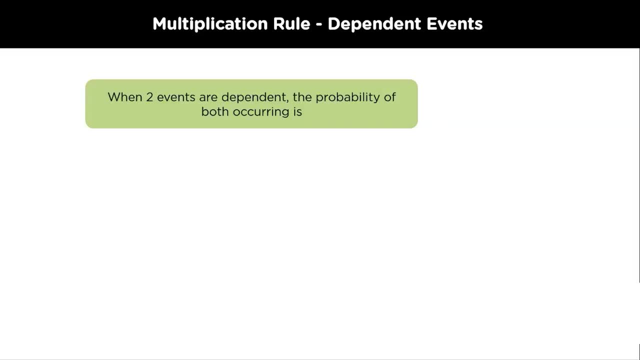 When you park at a no parking zone, the probability of getting a ticket increases. There is a multiplication rule associated with the dependent events. It says that when 2 events are dependent, the probability of both occurring is given by this formula, which is: P is equal. 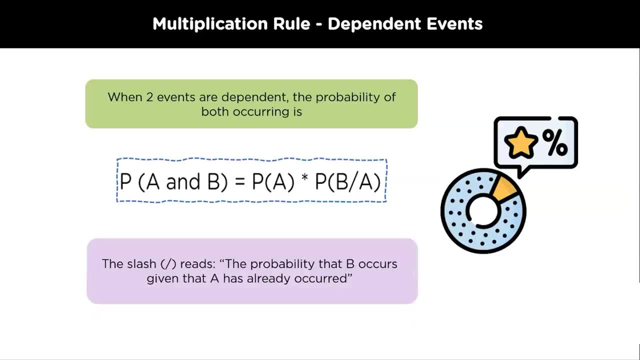 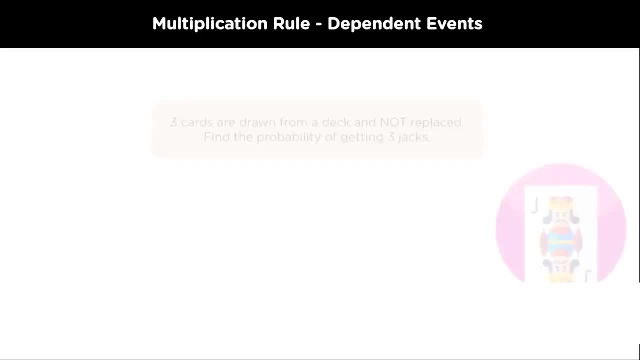 to P: probability of A into probability of B, slash A. The slash reads the probability that B occurs, given that A has already occurred. Let's look at an example: 3 cards are drawn from a deck and are not replaced. What will be the probability of getting 3 jacks? So 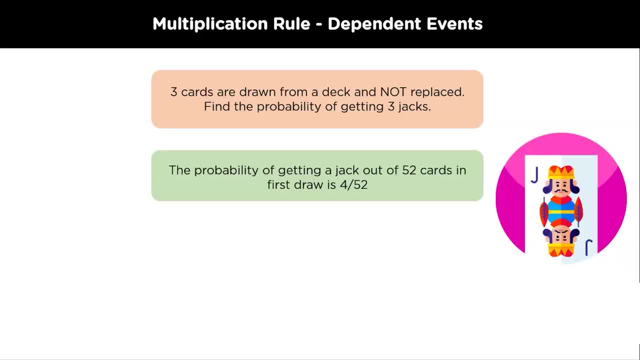 of getting three jacks. So in this case, the probability of getting a jack out of 52 cards in the first draw will be 4 by 52.. Now, after we have drawn the first card, there are 51 cards left. The probability of getting a jack in a. 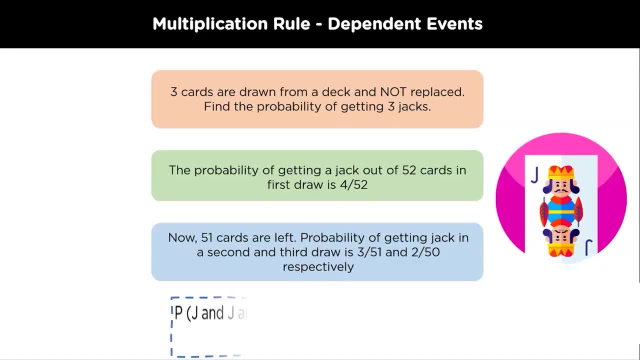 second and third draw will be 3 by 51 and 2 by 50 respectively. So according to the formula, the probability of getting the three jacks will be P0.76 into 0.58 into 0.04 will come up to be 0.00176. Now that we know. 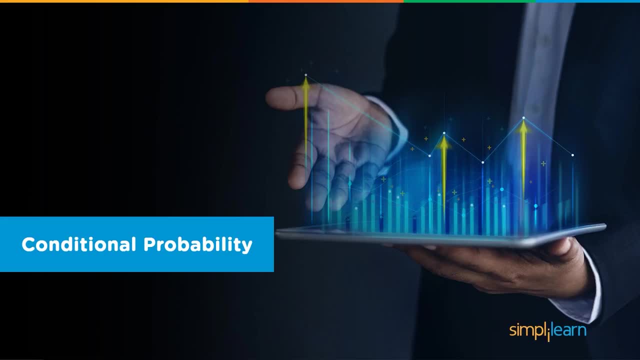 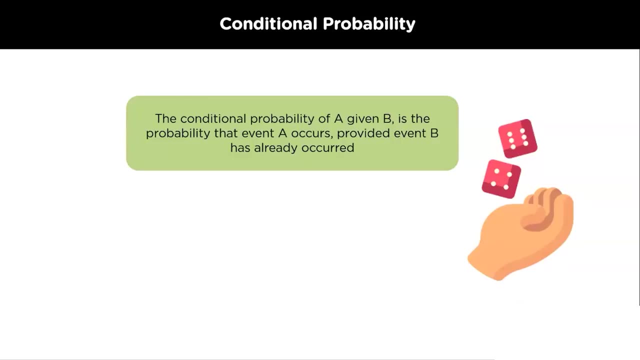 all the basic concepts in probability theory, we'll move on to conditional probability. Let A and B be the two events associated with a random experiment. Then the probability of A's occurrence under the condition that B has already occurred is called the N provides 25.. 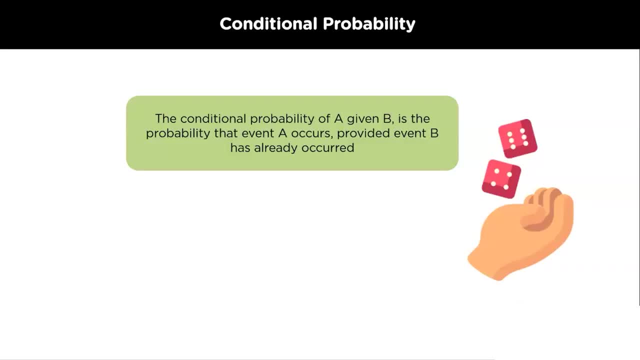 conditional probability. It is denoted by PA slash B. Thus we have: PA slash B is equal to PA intersection B divided by P. PA slash B is read as probability of occurrence of A, given that B has already occurred. Similarly, PB slash A can be called as probability of. 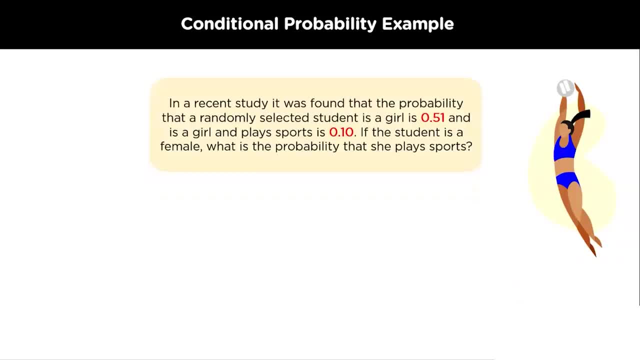 occurrence of B, given that A has already occurred. Let's look at an example. In the recent study, it was found that the probability of a randomly selected student is a girl is 0.51, and is a girl and plays sports is 0.10.. So if the student is a female, what is the probability? 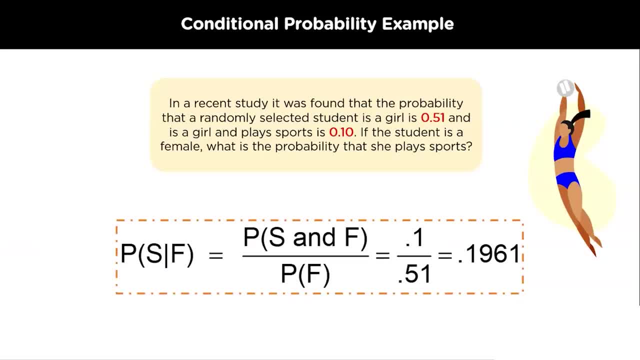 that she plays sports. In this case, the probability that the student is female and plays sport is 0.1, and the probability that the student is female is .51.. So the probability that student plays a sport, given that she is a female, will be 0.1 divided by 0.51, which will 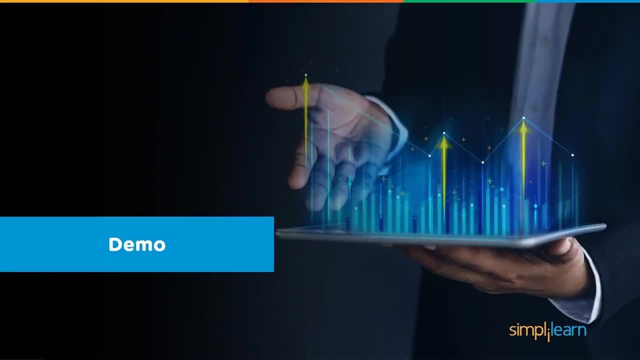 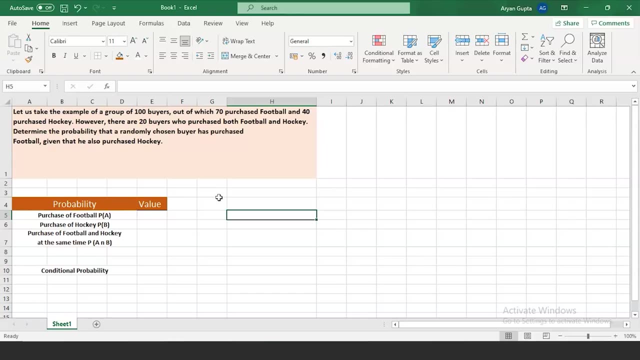 come out to be 0.1964.. Thank you. Now that we are done with all the theories related to conditional probability, we will move on to the demo in excel. Let's look at this problem statement. Suppose there are a group of 100 buyers, out of which 70 purchased football and 40 purchased 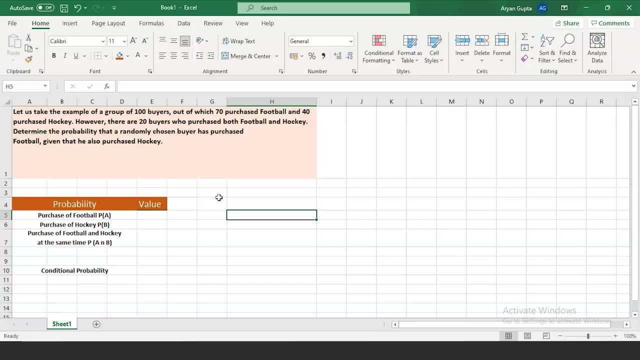 hockey. However, there are 20 buyers who purchased both football and hockey Determine the probability that a randomly chosen buyer has purchased football, given that he also purchased hockey. So this is a clear example of a conditional probability. Let's fill in this table. 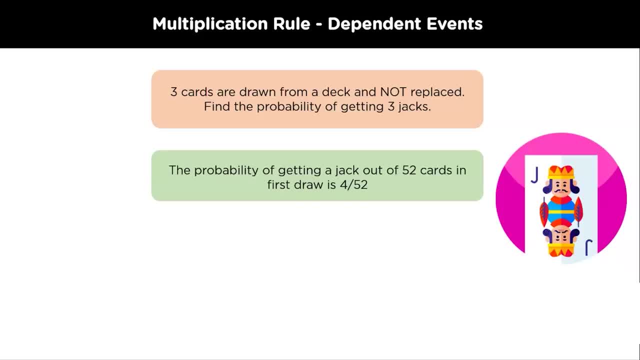 in this case, the probability of getting a jack out of 52 cards in the first draw will be 4 by 52.. Now, after we have drawn the first card, there are 51 cards left. The probability of getting a jack in a second and third draw will be 3 by 51 and 2 by 50 respectively. 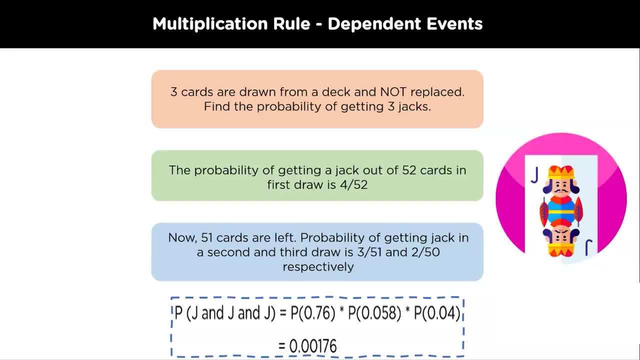 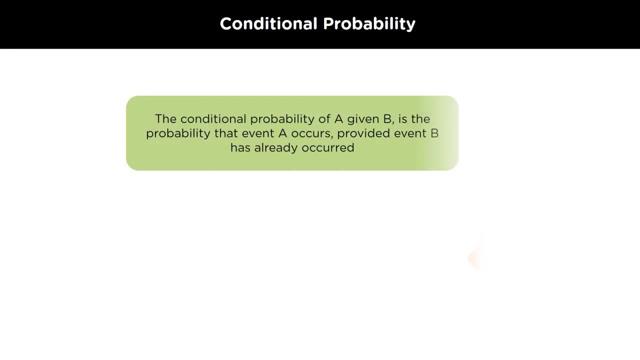 So, according to the formula, the probability of getting the 3 jacks will be P: .76 into .058 into .04 will come out to be .00176.. Now that we know all the basic concepts in probability theory, we will move on to conditional probability. Let A and B be the two events. 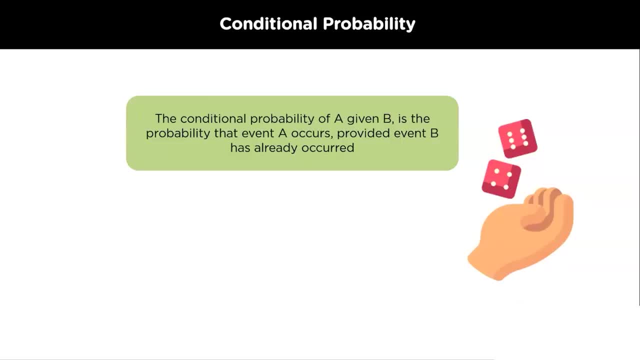 associated with a random experiment, Then the probability of A's occurrence under the condition that B has already occurred will be 0. is called the conditional probability. It is denoted by PA slash B. Thus we have: PA slash B is equal to PA intersection B divided by P of B. PA slash B is read as probability. 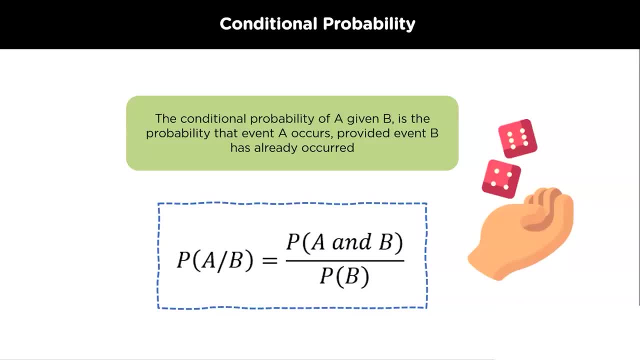 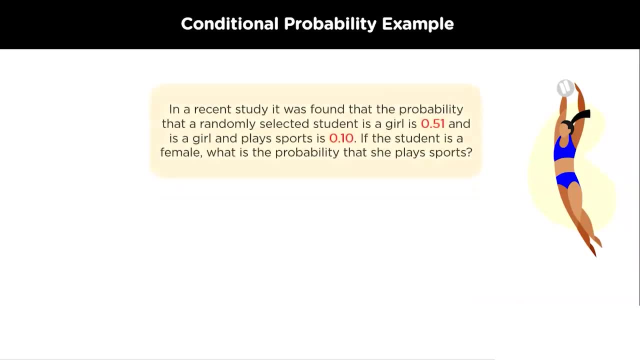 of occurrence of A, given that B has already occurred. Similarly, PB slash A can be called as probability of occurrence of B, given that A has already occurred. Let's look at an example. In the recent study, it was found that the probability of a randomly selected student 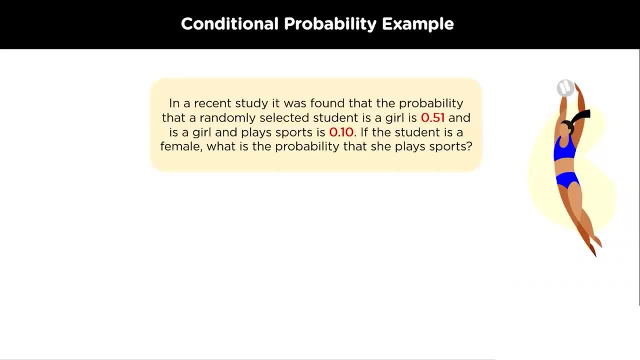 is a girl is 0.51, and is a girl and plays sports is 0.10.. So if the student is a female, what is the probability that she plays sports? In this case, the probability that a student is female and plays sport is 0.1 and the probability that a student is female is 0.51.. So the 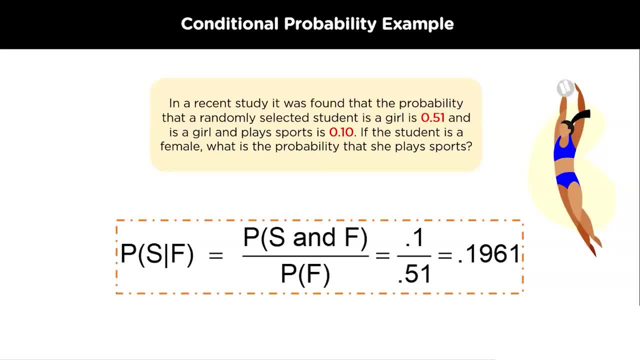 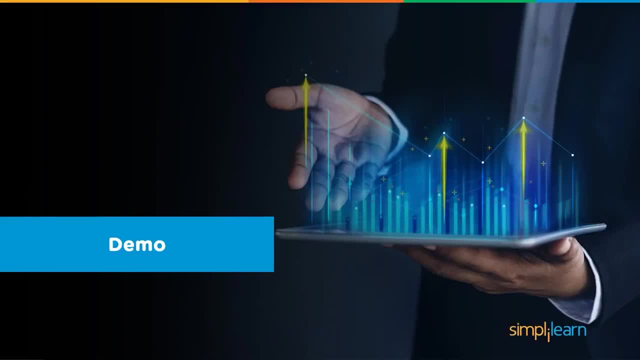 probability that a student plays a sport, given that she is a female, will be 0.1 divided by 0.51, which will come out to be 0.1961.. Now we are done with all the theories related to conditional probability. We will move on to the demo in excel. 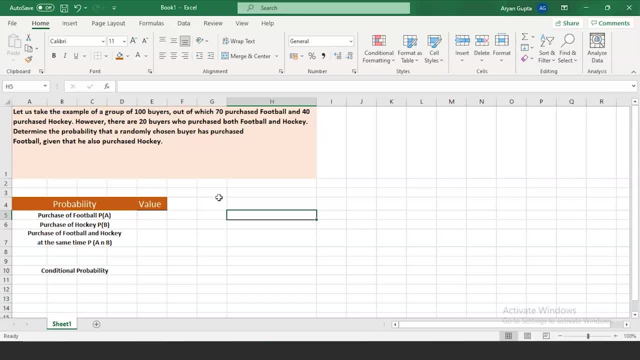 Let's look at this problem statement. Suppose there are a group of 100 buyers, out of which 70 purchased football and 40 purchased hockey. However, there are 20 buyers who purchased both football and hockey. Determine the probability that a randomly chosen buyer has purchased.